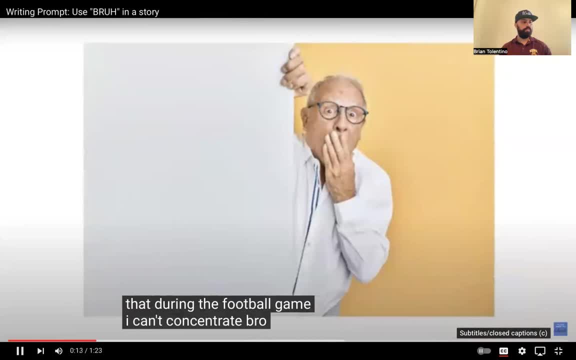 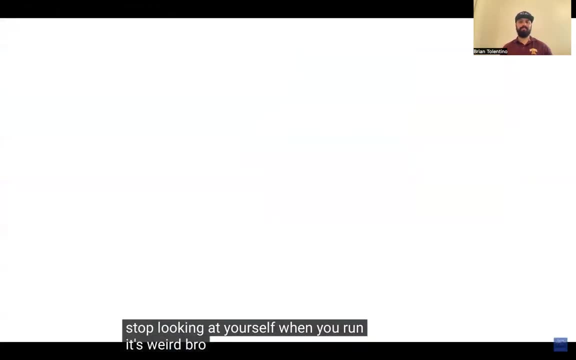 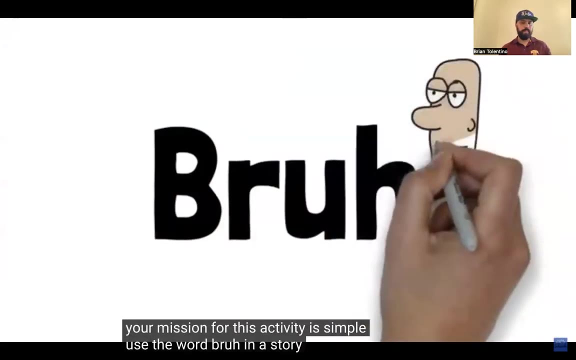 like that during the football game. I can't concentrate, bro. Bro, stop looking at yourself when you run. It's weird, bro. Your mission for this activity is simple: Use the word bro in a story. You can use it once, twice or ten times, Just be sure you use the word. 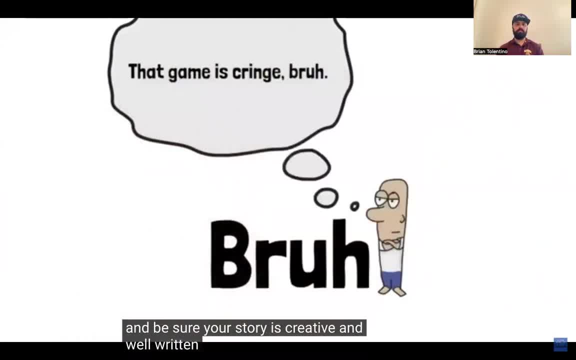 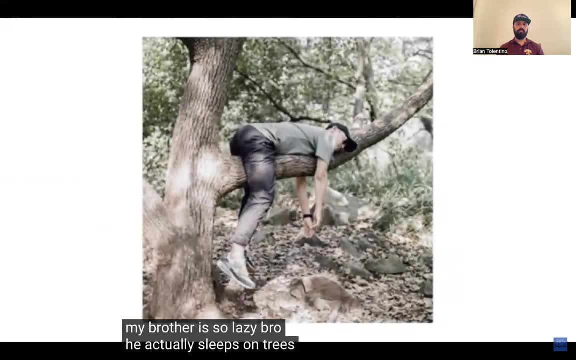 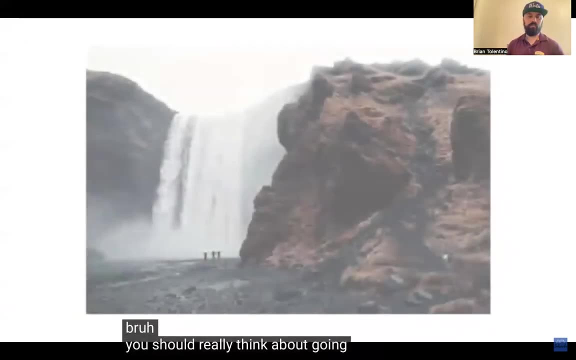 bro, Be sure your story is creative and well-written. bro, My brother is so lazy bro, He actually sleeps on trees. Can you take those glasses off your dog, bro? Bro, you should really think about going to Iceland. The place is lit, bro. Do you know what the best food in? 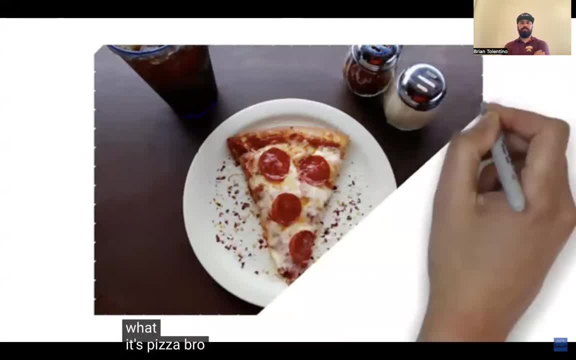 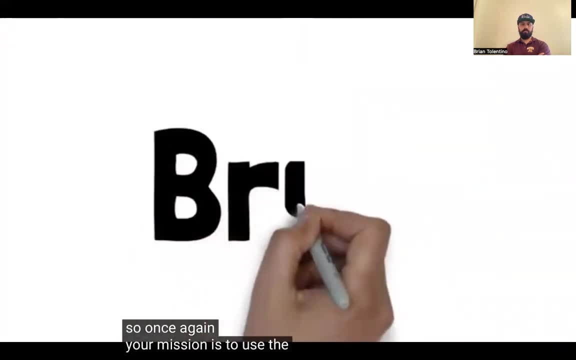 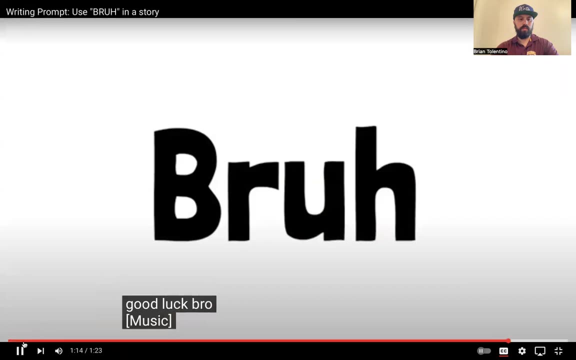 the world is. It's pizza, bro. Pizza is so good. So once again, your mission is to use the word bro in a story. Good luck, bro. All right. So I really like this prompt, And let me explain how I do this. So I have. 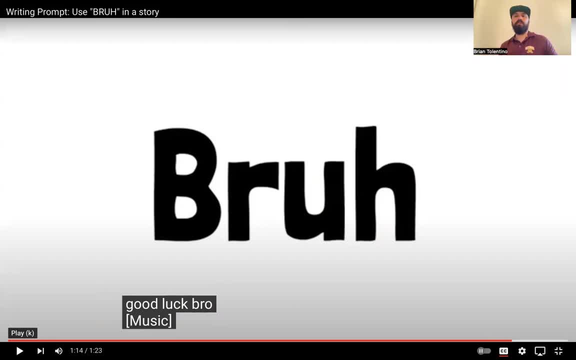 a creative writing prompt. I tell students: hey, we're going to write a story using the word bro, And they're always like what We're like. yes, We're going to use the word bro. I'm going to show you the video explaining it And then I show them. 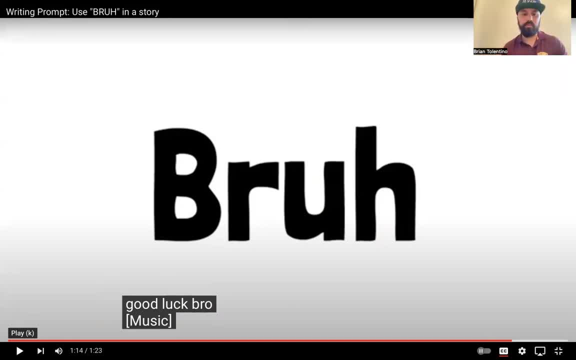 Okay, And then what I'm trying to do with this creative writing prompt is I'm trying to I want students to build the habit of sound writing, And by sound writing what I mean is I'm trying to set students up for later on when we write formal essays, Because 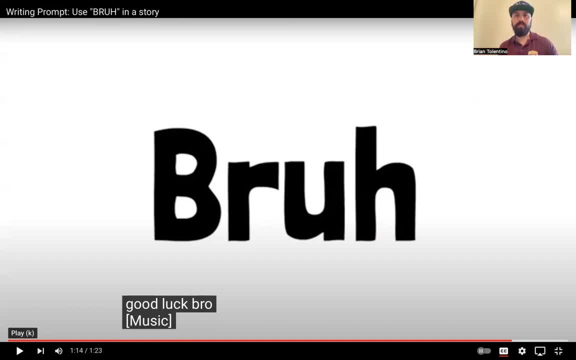 one problem I run into a lot with student writing is the sentences aren't right, the grammar isn't right, the punctuation isn't right, And then when we try to do an essay, it's just, it's just too much. The students get overwhelmed and you can lose them. right? I'm trying to. 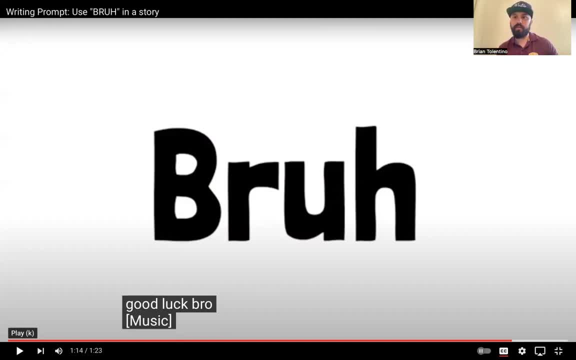 build- I'm trying to build- the habit of sound writing, clear sentences, proper punctuation, proper grammar, right. And that's what creative writing prompts really. it gives you the foundation of writing well, Because A when you use creative writing prompts, you're not stumbling over. 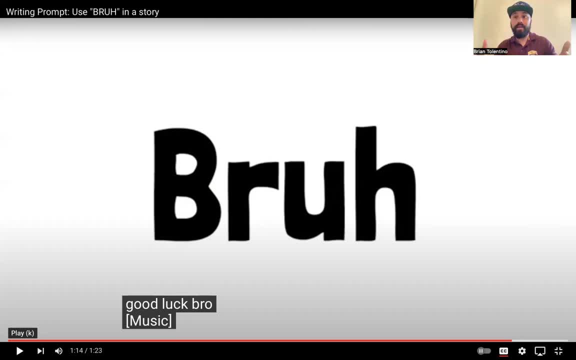 ideas. You're injecting your own personality and your own ideas into your writing Right. So me as the teacher, my goal is to try to teach the student how to harness these ideas with punctuation, grammar and clear thinking right. I tell students you can. 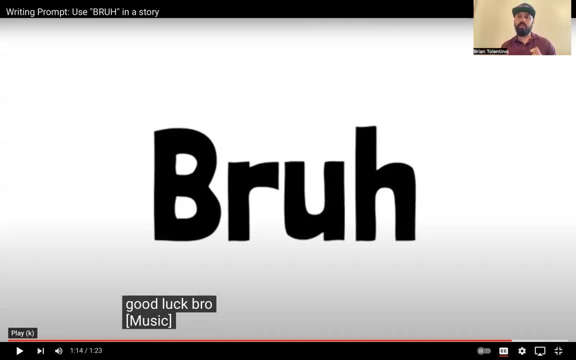 have the greatest ideas in the world, but if you don't write it clearly and if you don't use periods- and the writer doesn't- the reader doesn't understand what you're writing- those ideas are going to be lost. Okay, So that's what I really use these creative writing prompts for. 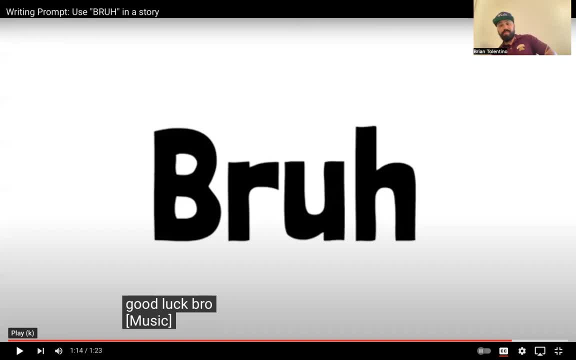 I I build upon the ideas and creativity of my student and I teach them how to harness those ideas we are writing. So what I'm going to do now is I'm going to show you an example, an example writing response to this And the student. what the student did in this response is the student. 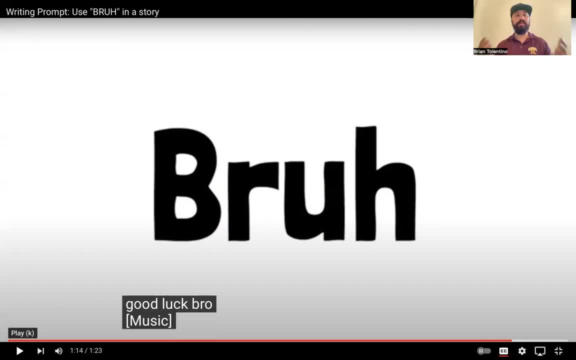 I noticed right away the student had really clever, imaginative, creative ideas, but the punctuation wasn't there. I mean, the punctuation wasn't there, The clarity wasn't there. So I sat down with the students and I built upon the positives. Hey, your ideas are funny. 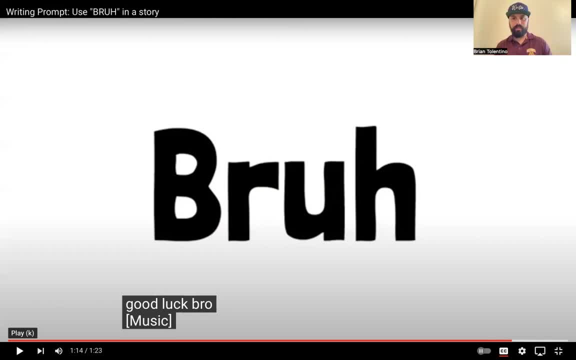 They're great, They're imaginative. Now let's figure out how to make this more clear. So we put periods in certain spots, We changed the word order of a certain things And I modeled that to the student to create the following example. So let me show you a student. 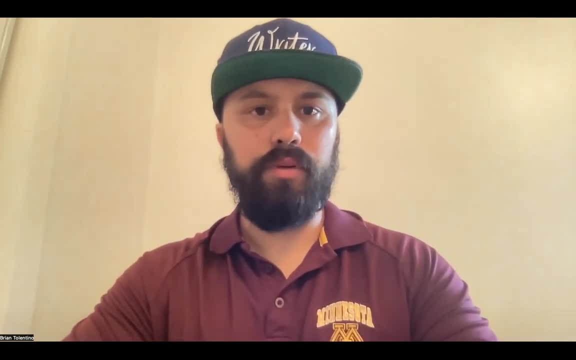 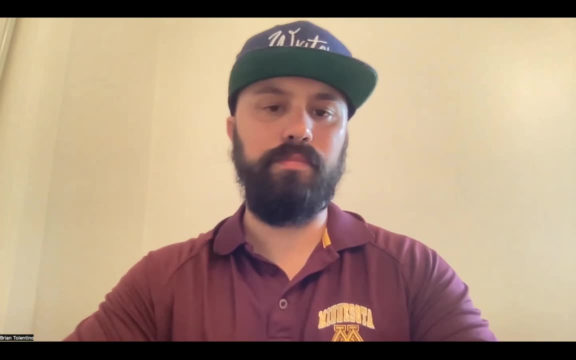 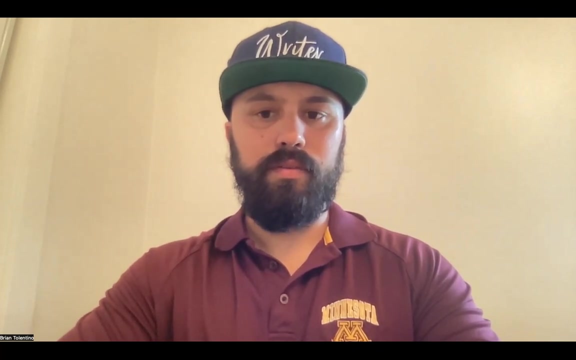 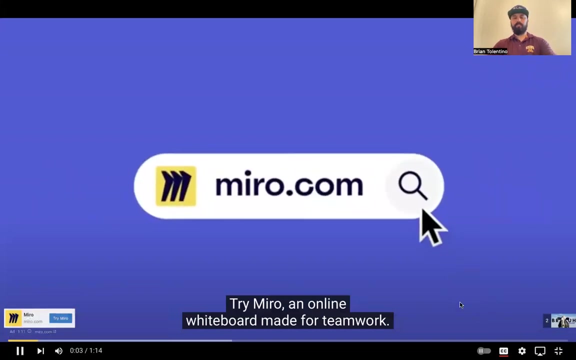 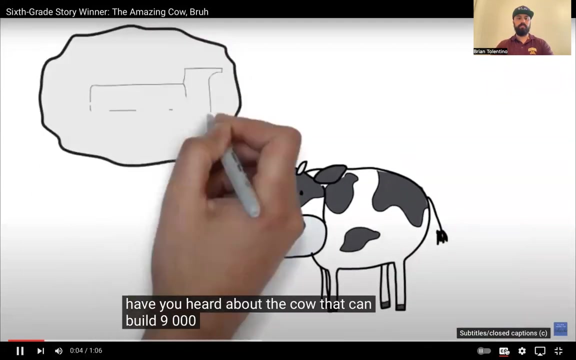 example to this response And I really love this. I love, I love, I love what he wrote: Searching for a better way to collaborate with your team. Here we go: An online whiteboard made for bro. Have you heard about the cow that can build 9,000? 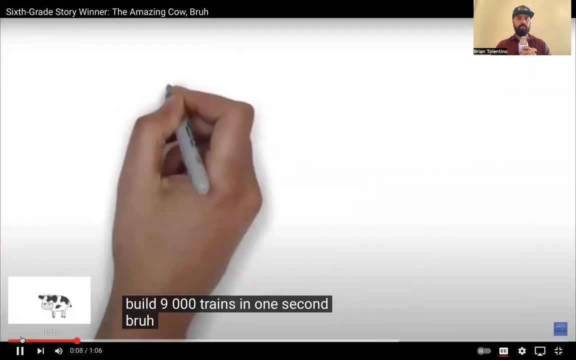 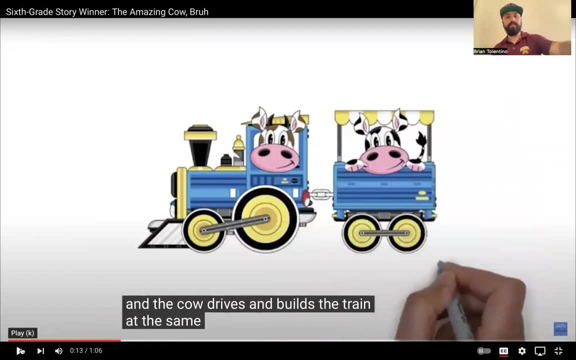 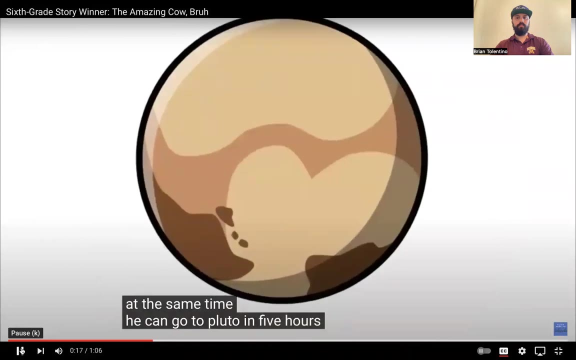 trains in one second. The train always passes inspection and the cow drives and builds the train at the same. This was written by a sixth grader. He can go to Pluto in five hours And the train only uses one gallon of water. And the train only uses one gallon of water And the 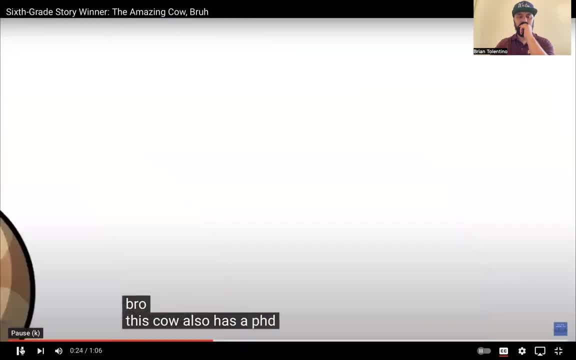 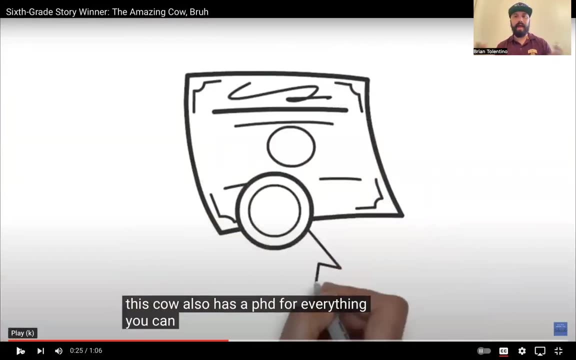 train only uses one gallon of gas. Bro, This cow also has a PhD for everything You can. So, um, when I was helping the student edit his writing, I asked him: what is a PhD? Where did you hear about a PhD? And he just said: I I I heard about PhD at home. and I asked him: what is? 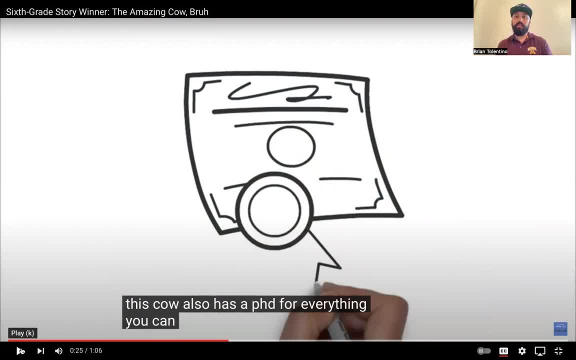 a PhD And he said it's like a professor. I said, yeah, you're right. So what we want to see students do is: they're taking notes, They're taking notes, They're taking notes, They're writing, And in their writing they're, they're conveying these ideas clearly And they're 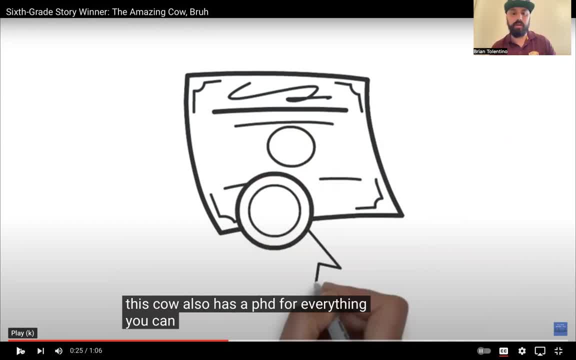 experimenting with these new words that they're using. This is what we want our students to be doing: Experimenting with language, taking ideas, injecting their own personality into their writing. This is exactly what I want to see, because the more you use these words, um. 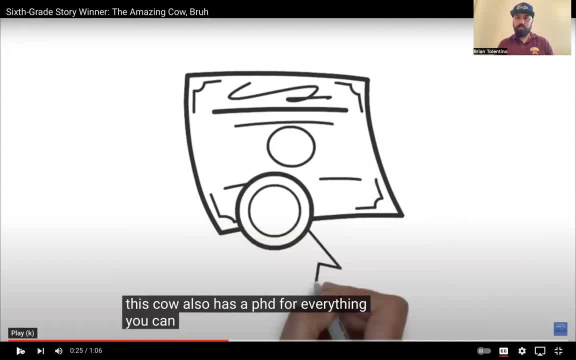 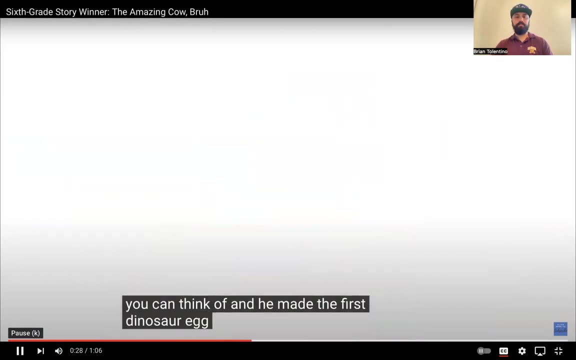 the better you're going to know how to use them. Uh, and once you start building momentum and you're learning new words and your writing's getting better, then it you learn other words and it just um, it's. it's good overall. So he made the first dinosaur egg of every species of. 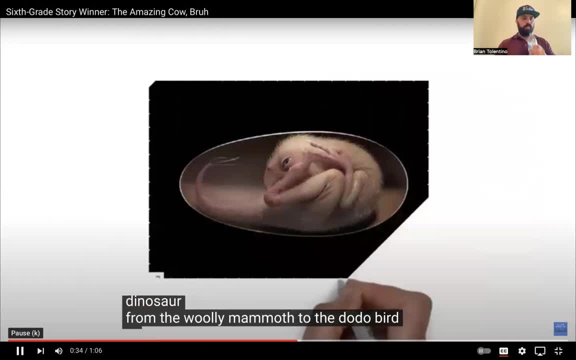 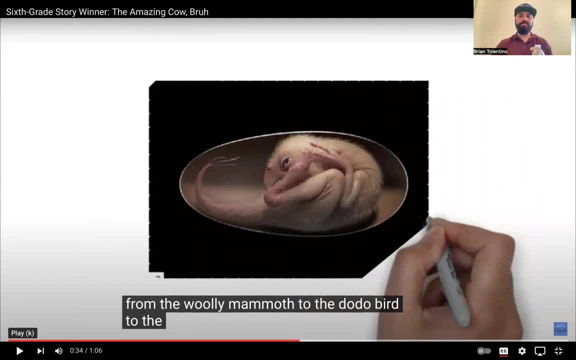 dinosaur, from the woolly mammoth to the dodo bird to the. so he's showing off. he's showing off what he knows, right. He knows about woolly mammoths, dodo birds, Thank you. He also discovered the. 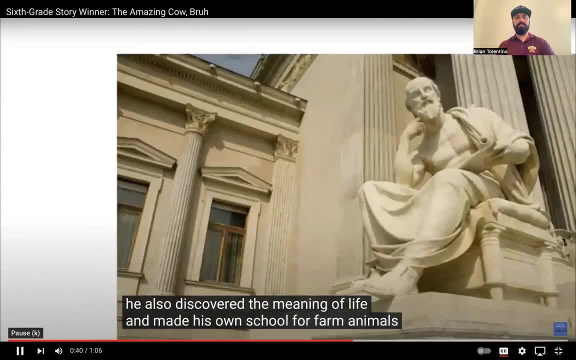 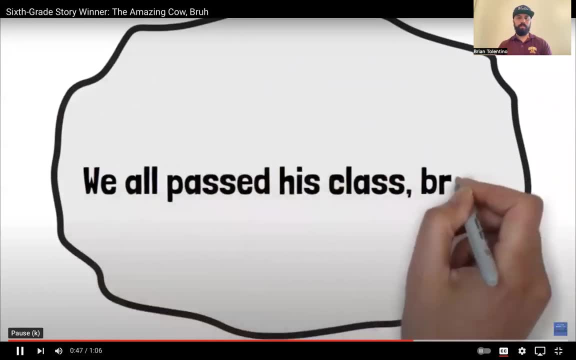 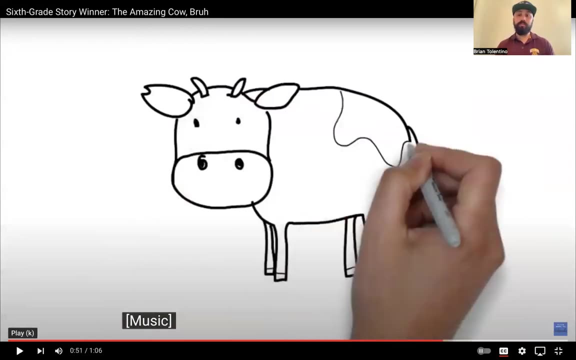 meaning of life, His own school for farm animals and all the animals always pass his class, bro, All right. So that's a student example. Let me see. That's a student example, not a long story. but this student isn't the fastest writer. Uh the. 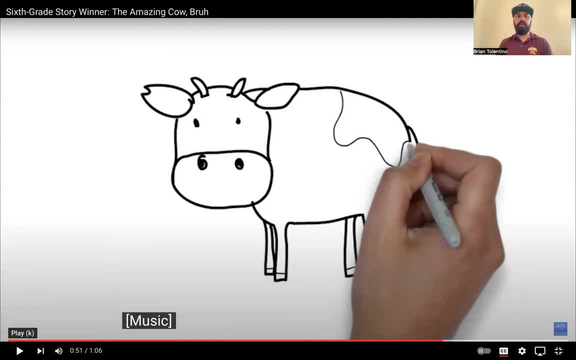 student. a lot of the had a lot of mistakes in his writing. Uh, but that's okay because, uh, I was able to build on his ideas And we were able to edit his writing and create a very clever and creative story that he can be.